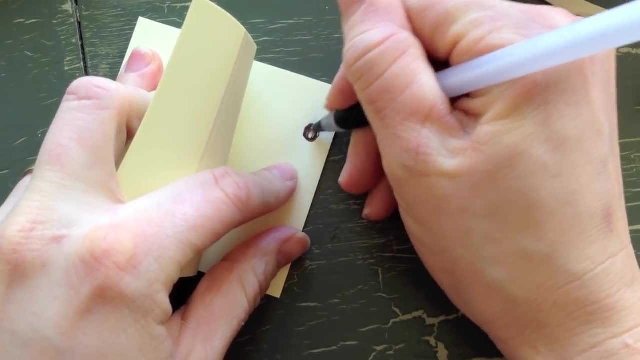 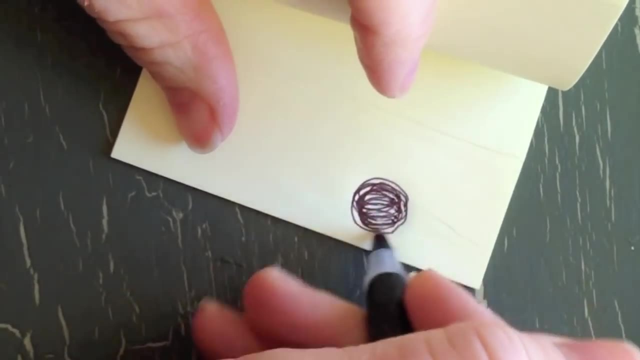 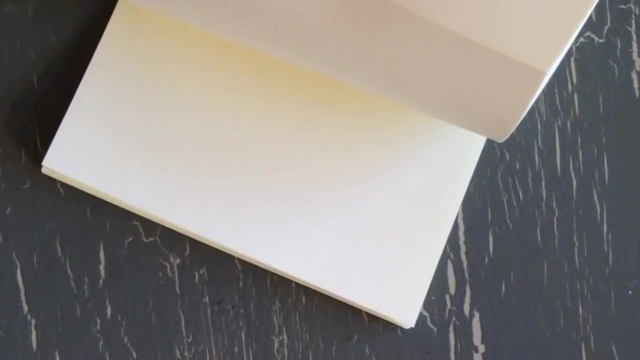 that way, I'm just going to slowly let it get bigger. This would have been easier with the marker. So my dot is moving from the side coming into the middle and it gets bigger. That is a good place to start. So I would just practice moving a dot across or, even easier, try moving. 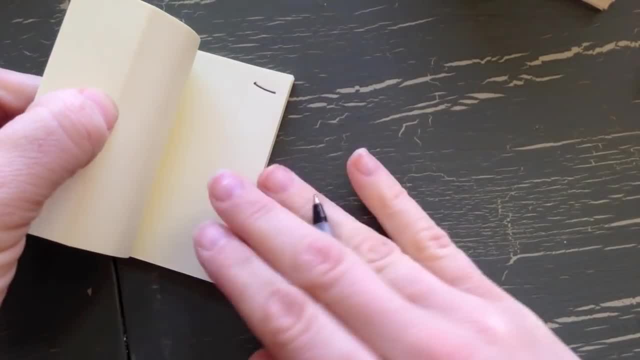 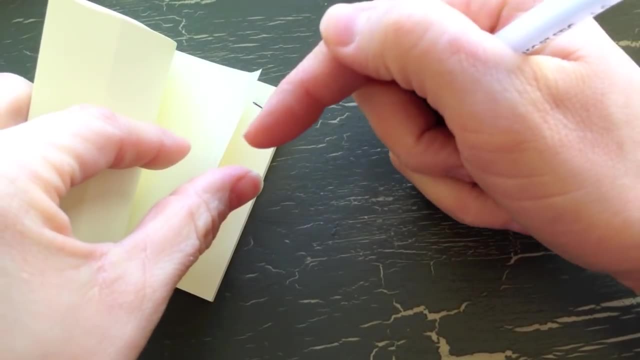 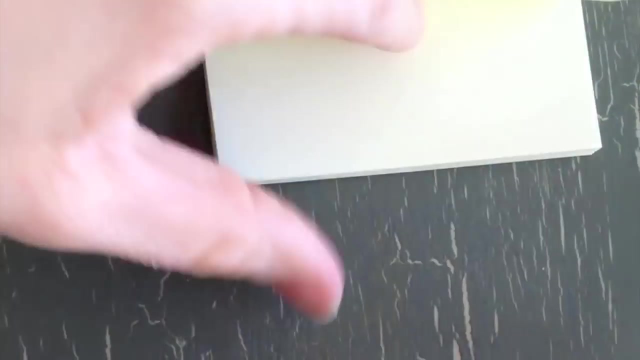 a little bit to the left and then move it to the right. So I'm going to go ahead and do that Line across. Just draw a line on the side, Get your next page down. So each time I'm moving it just a little bit in that direction. Now, when you draw your stick figure for this animation. 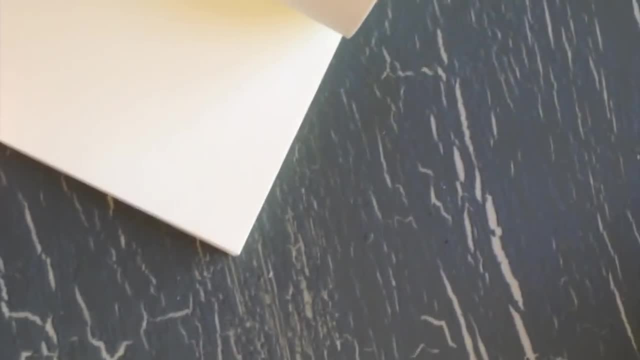 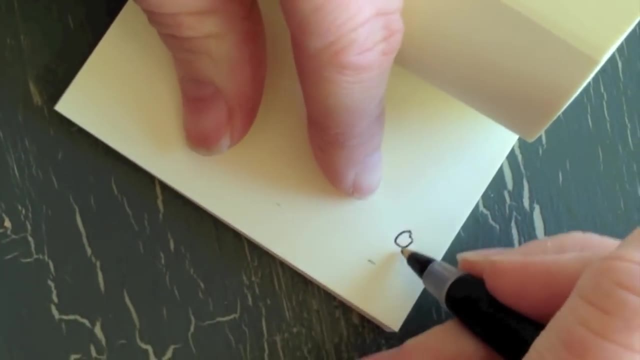 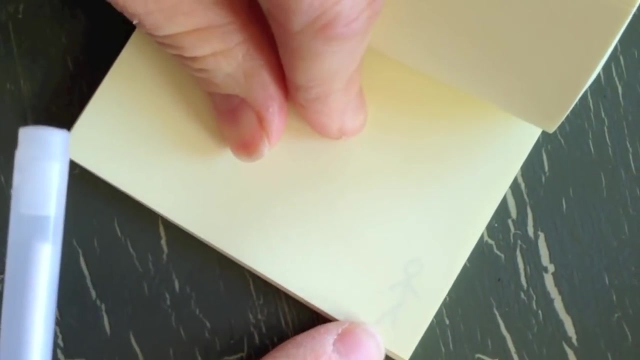 you can draw it any way you want. Start out with trying to make your stick figure jump, So I'm going to have him jump from here to the middle of my page. So here he is, Ta-da, With the next page over, so you can kind of see him through. Here is your person, They're. 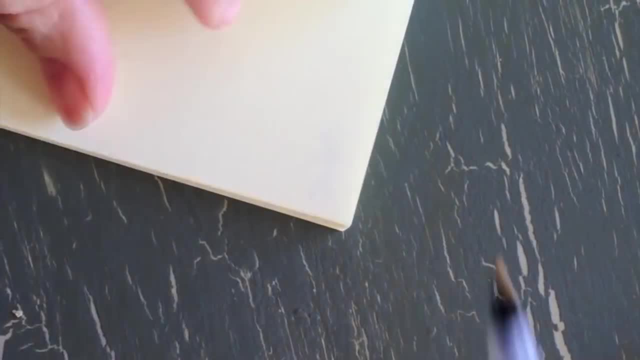 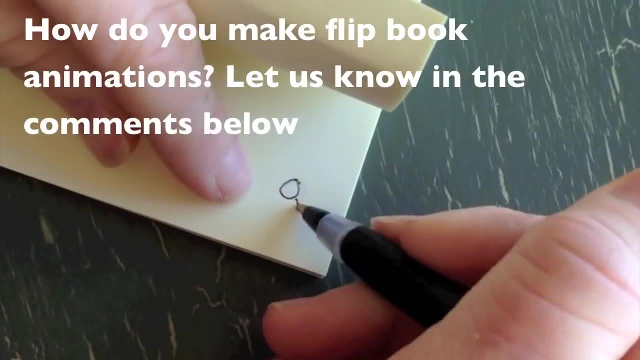 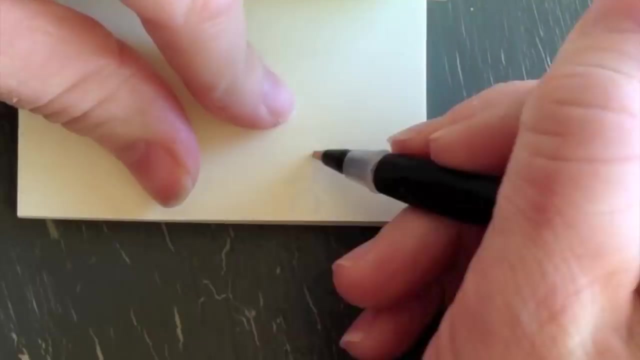 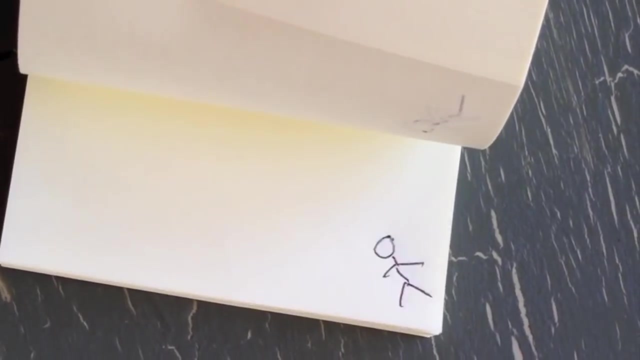 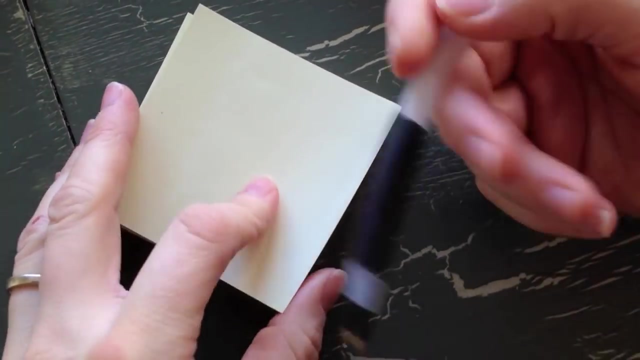 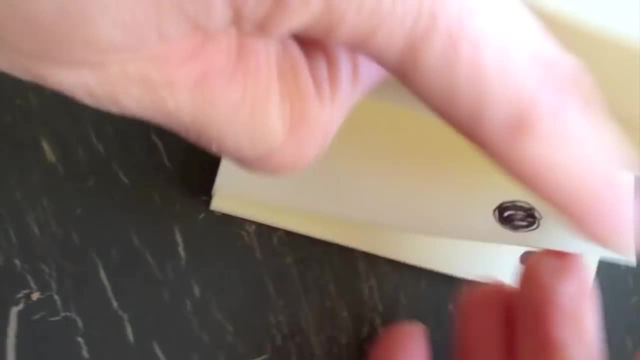 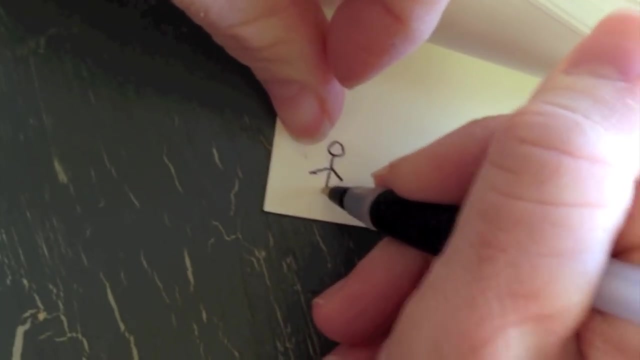 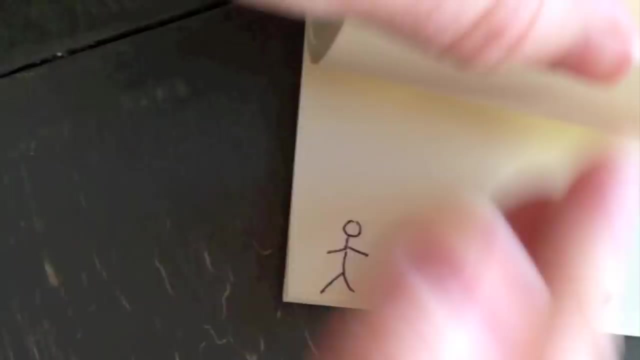 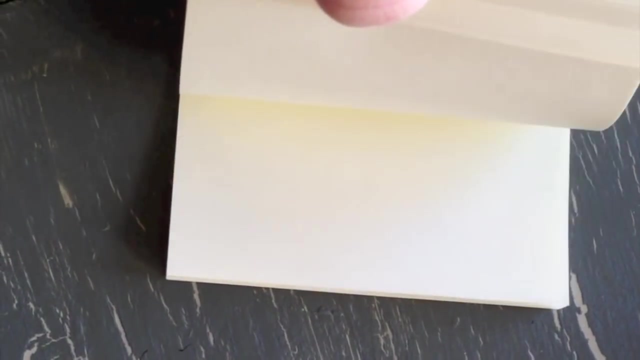 and do that. So I'm just going to start. in this corner There's my stick figure. Remember, I just flipped the next page so I can kind of see through where my drawing was before and it makes it a little bit easier to add the next step. Maybe we should make a stick figure that is waving. So